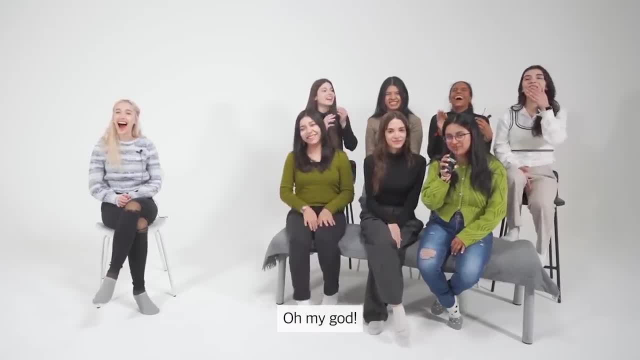 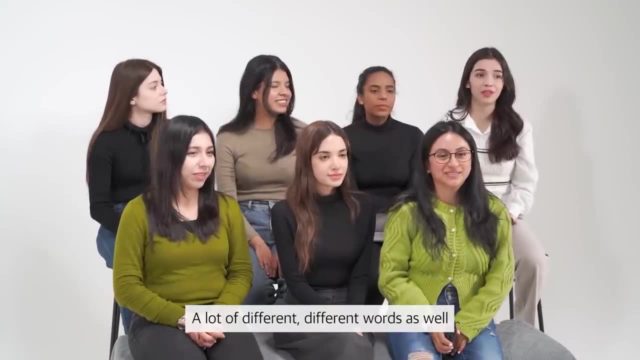 I don't think it's considered Spanish anymore. Oh my God, How do you know? No, it's because we have, like, different words, A lot of different words in that as well. Yeah, they use words in a whole different context. 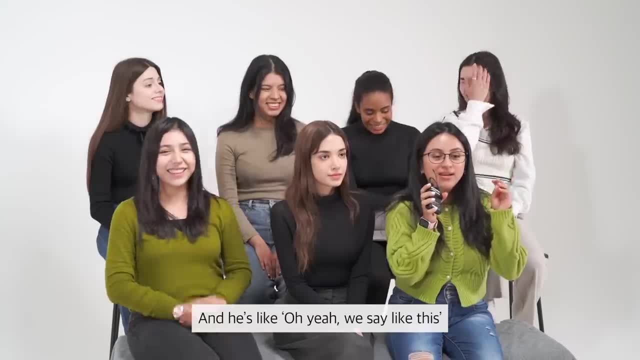 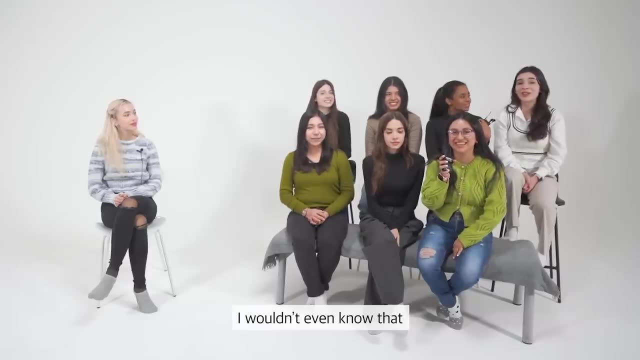 They have something about animals. I met a Chilean friend before And it's like: oh yeah, we say it like this. And I'm like: why are you using so many animal names for, like all of these type of situations? I don't even know that. 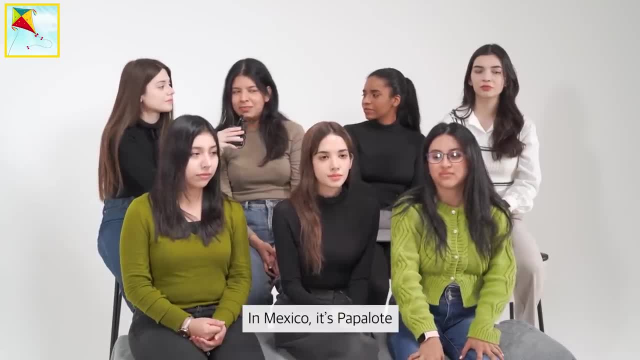 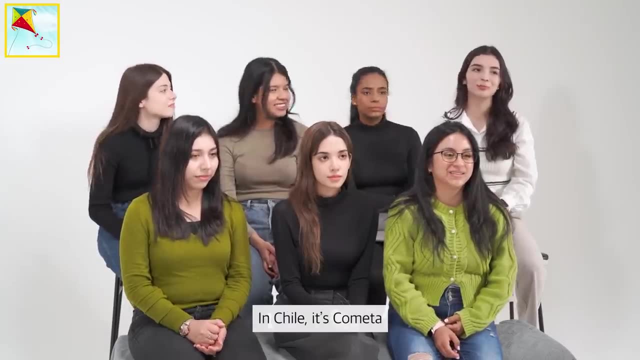 Okay, kite In Spain we say: cometa. In Mexico it's papalote, Papalote, Papalote, How cute. In Colombian also: cometa In Chile, it's cometa. In Peru, it's also cometa. 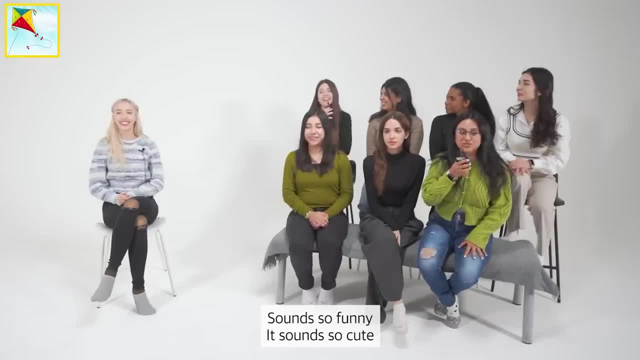 In Cuba it's papalote, In Ecuador it's cometa. It sounds so funny, It's so so cute And it's like has the word papa lote. It's like a lote of my papa. 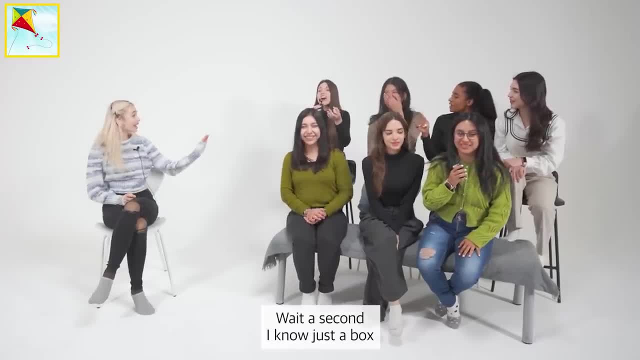 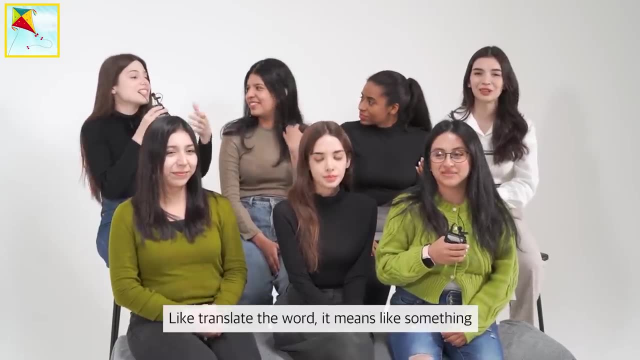 I don't know. It's papalote. Wait, wait. I don't know. It's just a box or something from my dad. I don't know It sounds. If you literally translate the word, it means like something from my dad. 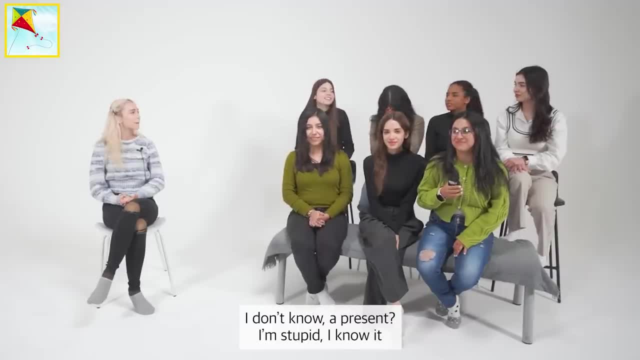 Like a lot Like a. I don't know, I'm stupid, I know it. To me it sounds like a parrot Papagayo. we say, Maybe like the colors, Maybe that's why I don't know. 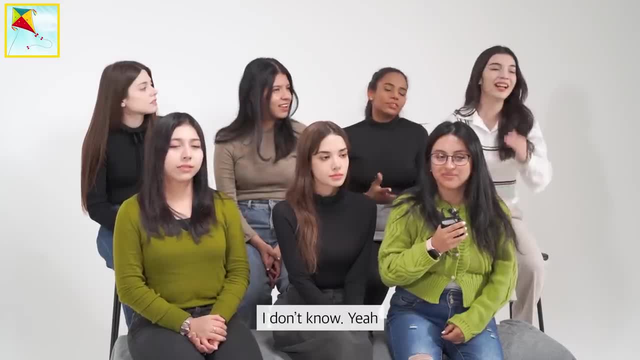 Maybe it's like a papagayo fly, but made of paper, I don't know. Oh my God, We would laugh so hard, but in a cute way. We would think it's really cute. Would you understand, though? No, 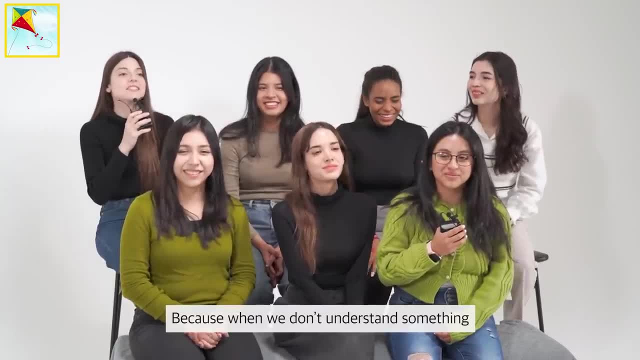 That's why We would laugh, because when we don't understand something, we don't want to show we're stupid, So we just laugh. and then we say, oh wait, What was that It's like? but we have to laugh first. 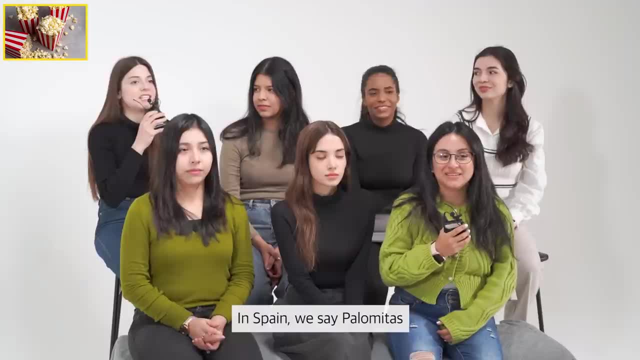 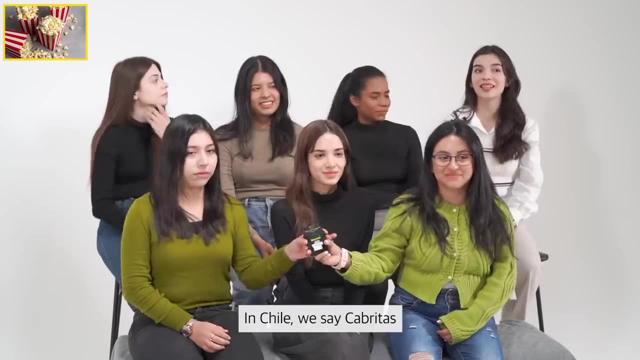 Popcorn. In Spain we say palomitas, Yeah. In Mexico, we say palomitas In Mexico, we say palomitas In Colombia, we say crispetas. In Chile we say cabritas. In Peru we say canchita. 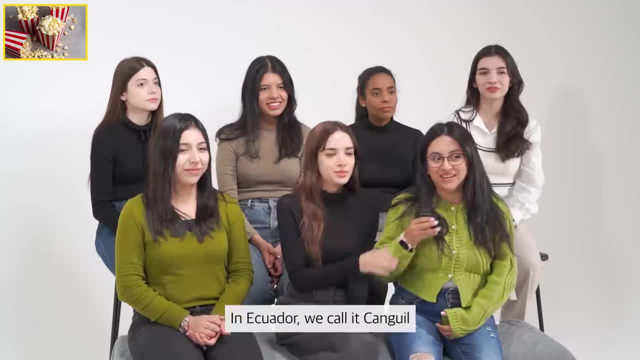 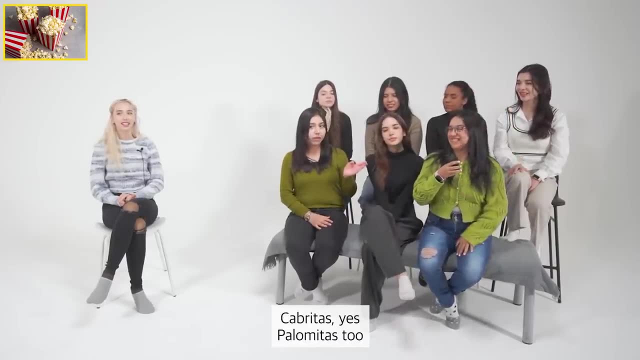 In Cuba we say rosa de maíz or rositas de maíz. In Ecuador we call it canguil. I heard of palomitas before, But you say cabritas, Cabritas, Cabritas. 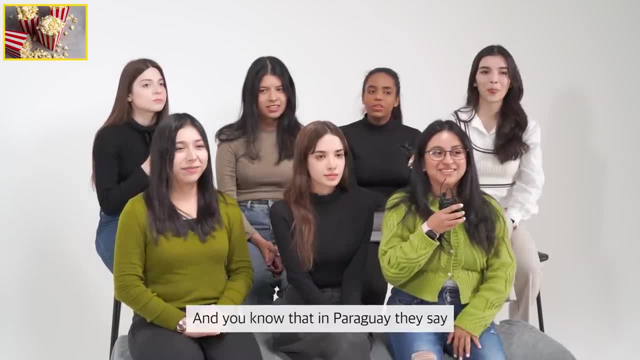 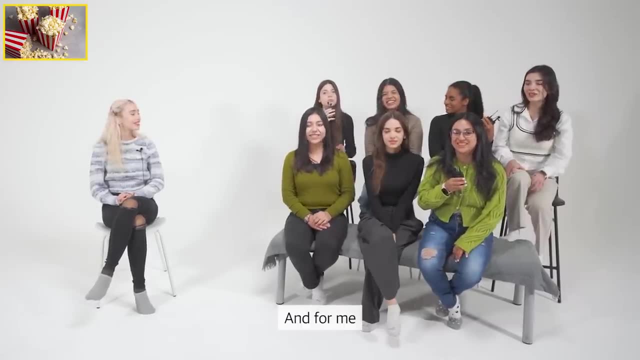 Cabritas- Yes, It's a lot of it, Cabritas. No, For us it's 100 percent canguil, And you know that in Paraguay they say pororo, Pororo, Pororo, Oh, pororo. 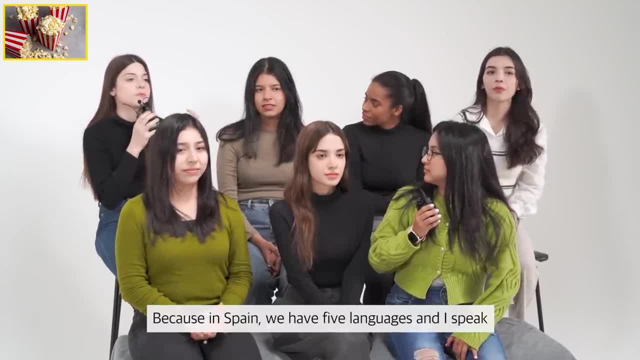 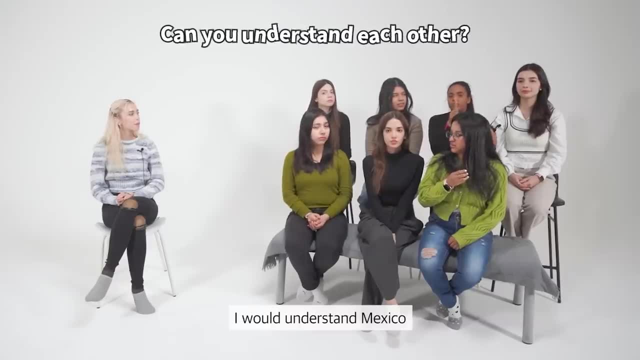 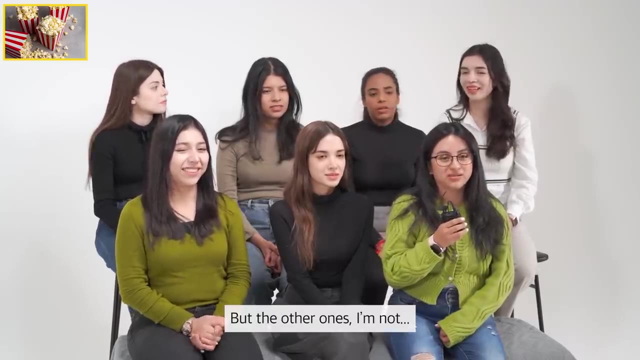 Yeah, It's really curious because in Spain we have five languages and I speak Catalan as well and we say crispetas. So it's quite similar. Maybe only palomitas. I would understand Mexico, Spain and maybe Cuba, because it's like very graphic, But the other ones I'm like 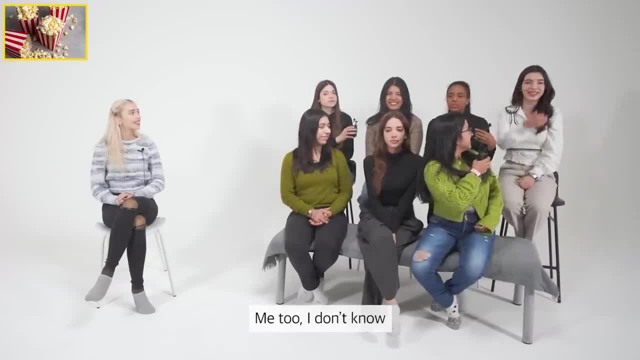 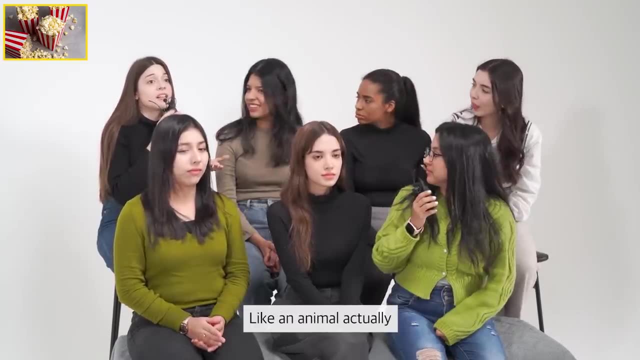 Can anybody understand Chilean? ¿Por qué cabritas? Me too, I don't know. I would think it's chicharrón or something like that. Chile cabritas sounds like an animal actually. You see, you see, Cabra, cabra, cabra. 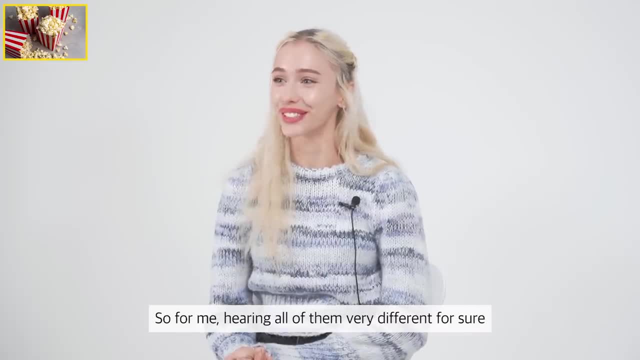 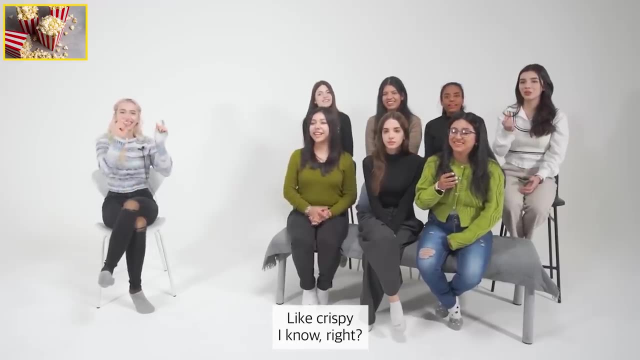 A little goat. So for me, hearing all of them very different for sure, But I think the one that makes the most sense in my English brain is probably like crispetas, Because it sounds like I'm crispy. I know right In Spain, cangrejo. In Mexico cangrejo, Colombia too cangrejo, Chile, jaiba. In Peru it's cangrejo, Cuba es cangrejo. In Ecuador it's also cangrejo. But when we want to buy like a bunch of crabs, we say jaiba. 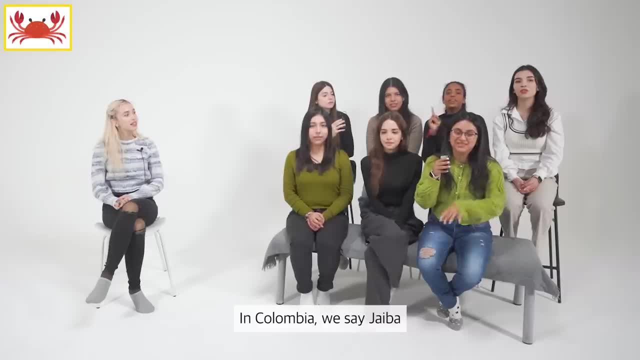 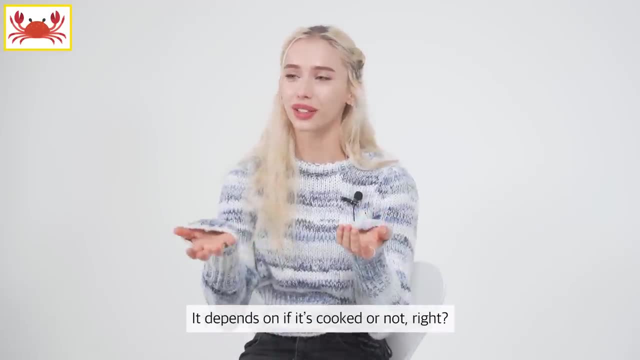 So we just use that word, but it means like a bunch of crabs. In Colombia we say jaiba only for like a dish made with cangrejo. Yeah, I was gonna say I think it depends on if it's cooked or not, right? 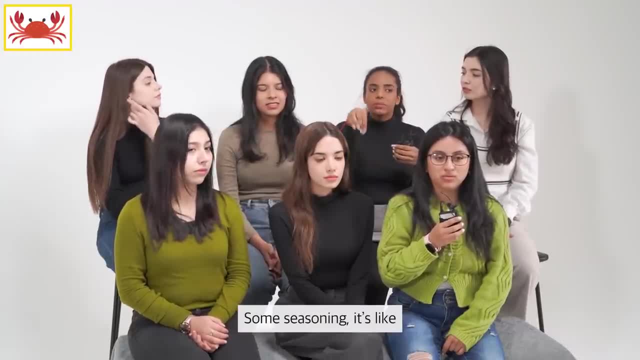 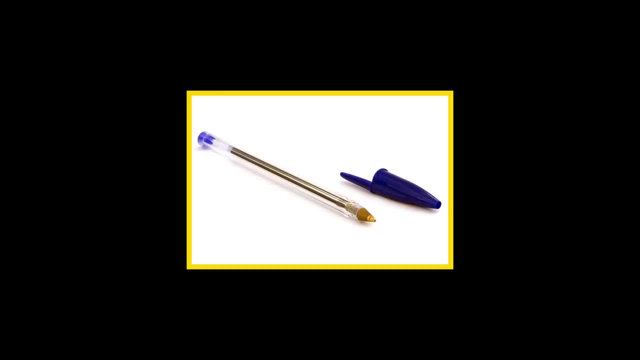 If it's the shell with the meat inside and some seasoning, it's like jaiba al, I don't know what style, But when you say the animal, it's just cangrejo. In the US we say pen, In Spain, boli In Mexico, pluma. 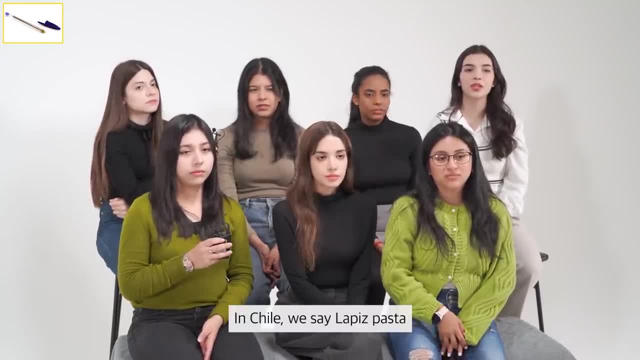 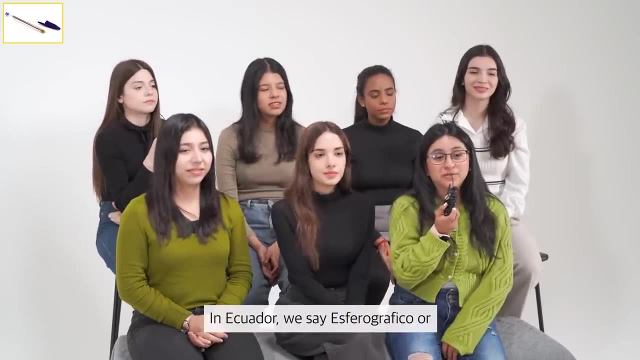 In Colombia we say lapicero or esfero. In Chile we say lapispasta. In Peru we say lapicero o bolígrafo. In Cuba we say pluma. In Ecuador we say esferográfico o esfero. Wow, so hard. 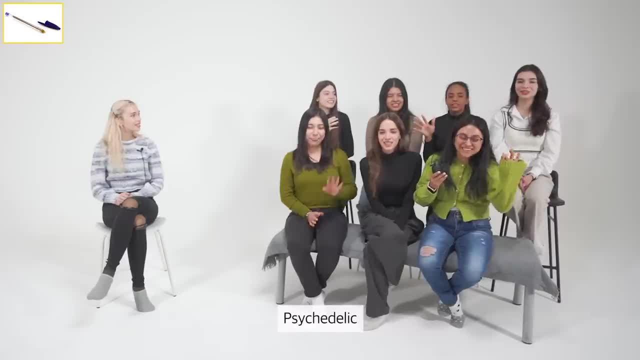 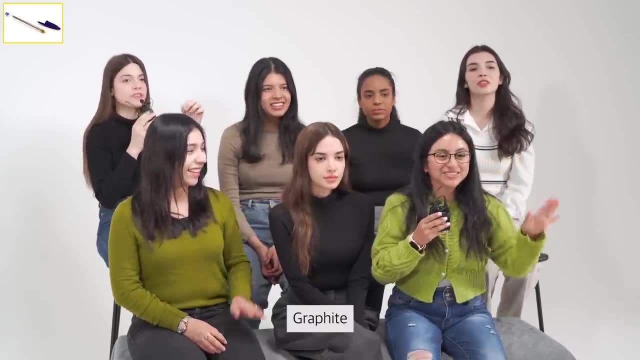 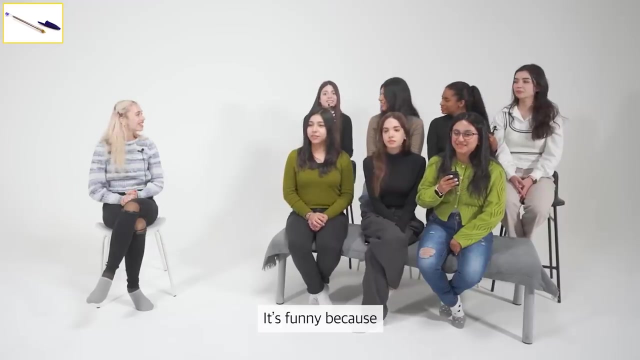 Wait, wait, wait. that sounds so psychedelic. It's kind of describing the shape. it's like this rounded graphic. Esferográfico sounds really like artistic. I don't know, But I'm most used to pluma. It's funny because for us in Spain, pluma means in the old times, when people eat. 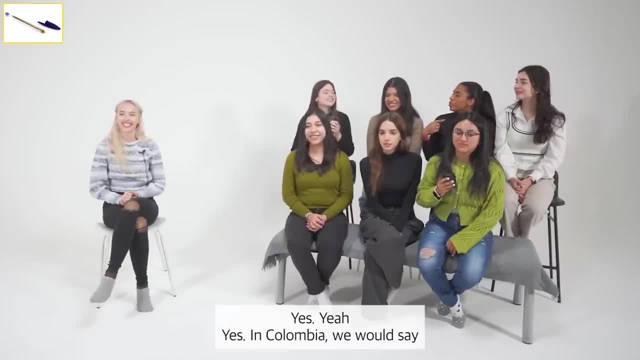 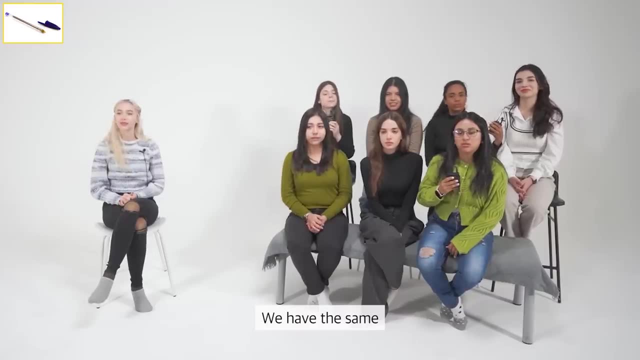 Yes, like the ink one. Yes, yes. In Colombia we say pluma or plumón, or when it's like the one with the ink Yes. yes, we still do have that one. we have the same Lapispasta pasta. yummy, Wow, pasta. 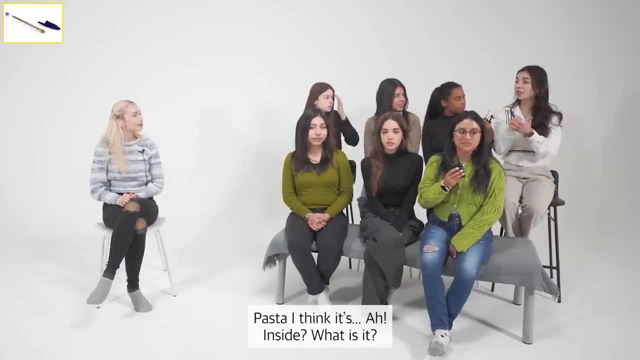 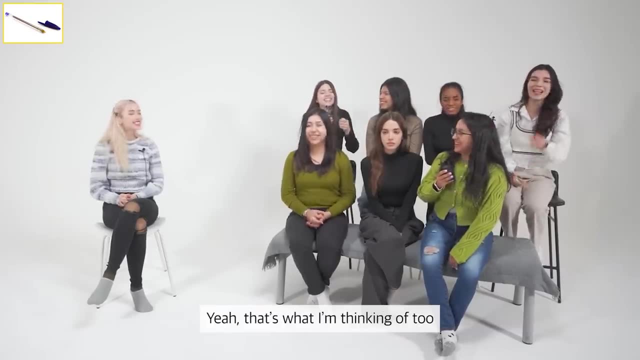 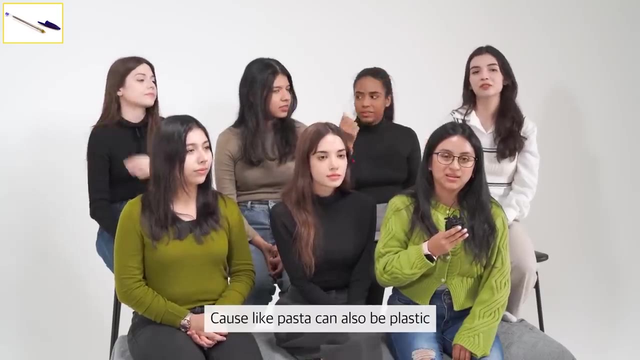 Pasta, I think, is in Thai. what is it? So we say pasta is in Thai, so lapis of pasta, I just think of spaghetti with a pen. I thought that it was like lapis but made of plastic pasta, Because like pasta can also be plastic. 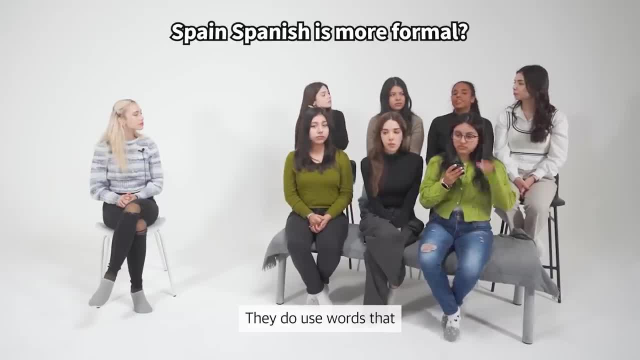 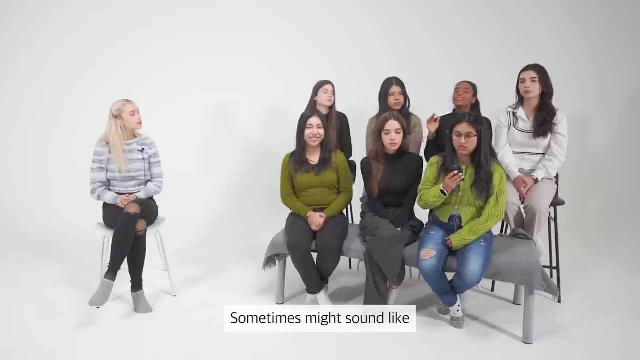 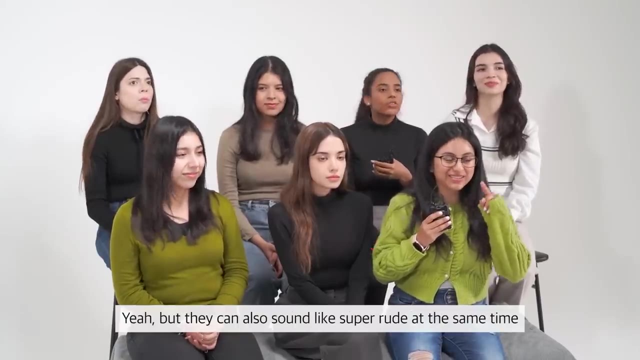 Makes sense. When Spanish people speak, they do use words, that old words, You know, like the words that we don't use on our daily lives. So they sometimes might sound like more formal when they speak, But they can also sound more rude. Yeah, but they can also sound like super rude. 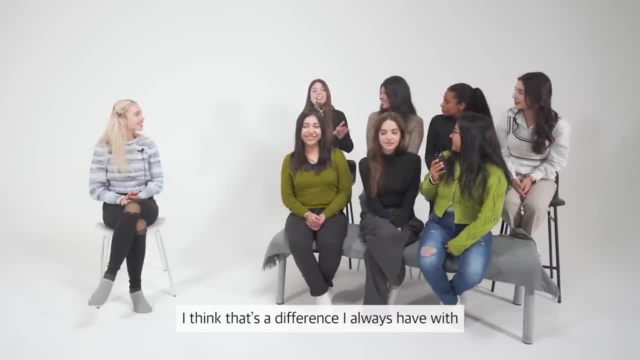 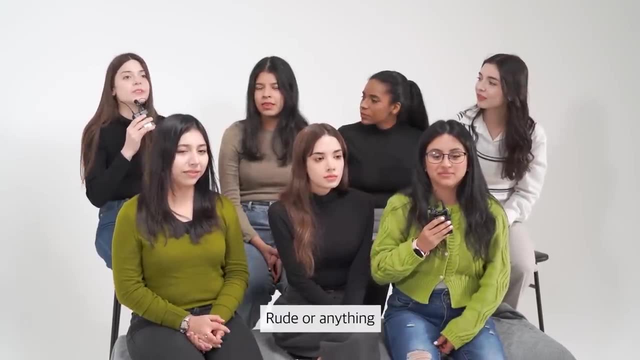 Not in Spain. I think that's a difference I always have with Latin American people. We use those words as well, and it's not even more formal or rude or anything. It's just up to your preference, and something like that. I think it's because it's more straight. 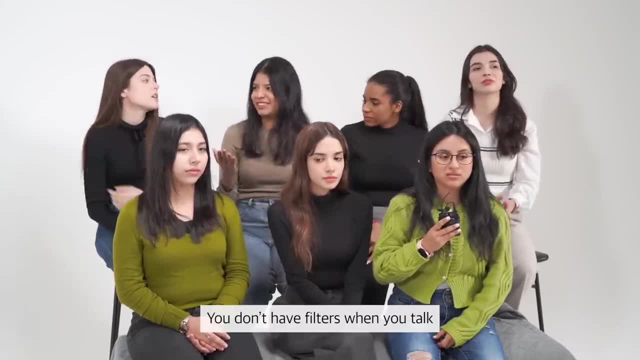 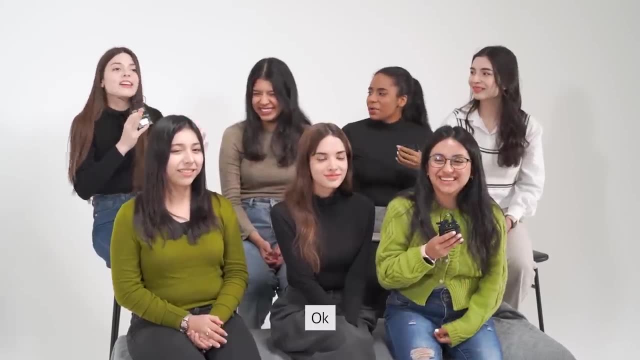 Maybe, So for us it's like you don't have filters when you talk. But you guys are all so soft and cute and already giving love to everyone And we are a little bit more okay. We are also energetic When you say like vosotros entendéis we? 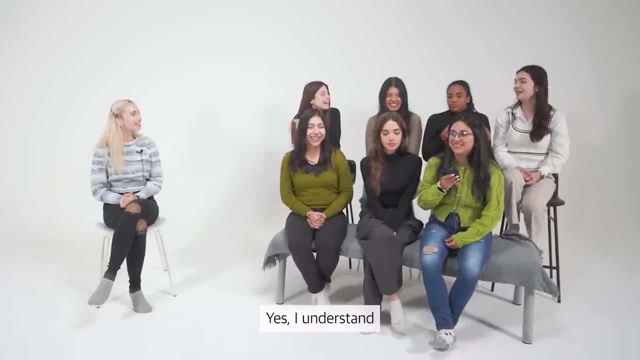 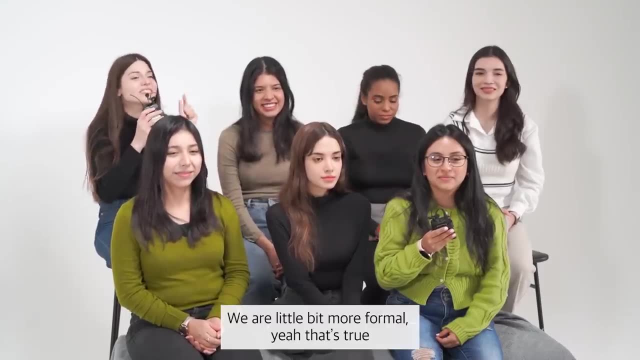 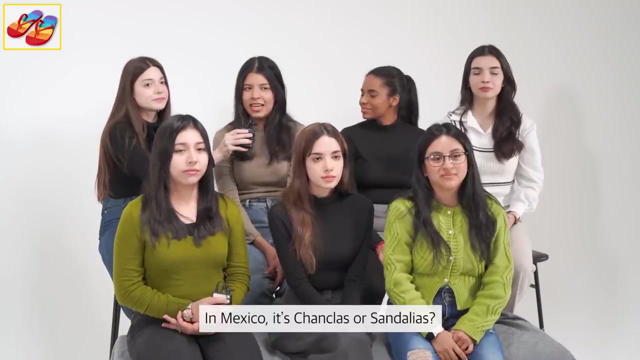 Yeah, we never use vosotros. Excuse me, ma'am. Yes, I understand, It sounds so formal. Yeah, Ma'am, We are a little bit more formal, that's true. We say flip flops In Spain, chancletas. In Mexico it's chanclas or sandalias. 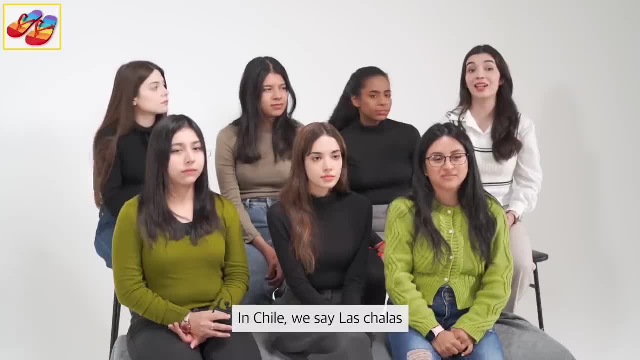 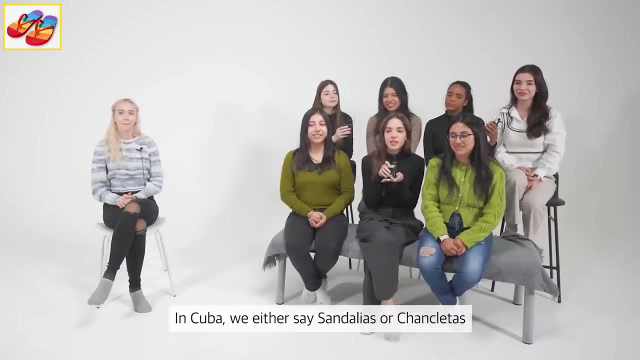 Basically the same, like chanclas. In Chile we say la chala La, what La chala La chala? In Peru, we also say sandalias or chanclas. In Cuba, we either say sandalia or chancleta. In Ecuador we also say sandalias or chanclas. 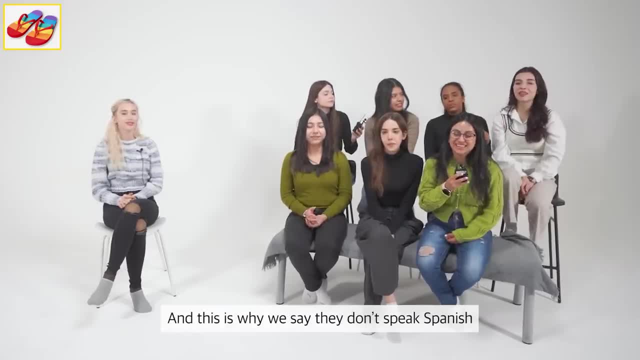 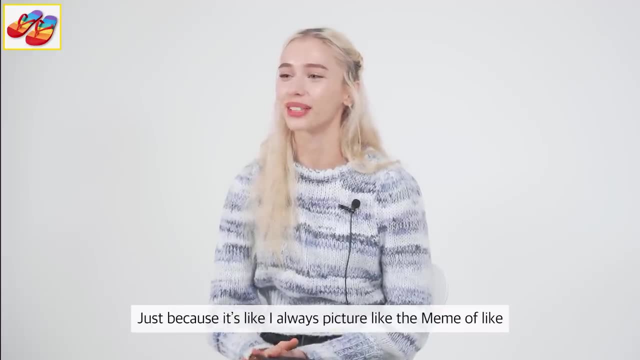 Right what happened With Chile, And this is why we say they don't speak Spanish. Si, I think so. I think, I think I like chanclas, Just because it's like I always picture, like the meme of, like the mom, Chancla, chancla. 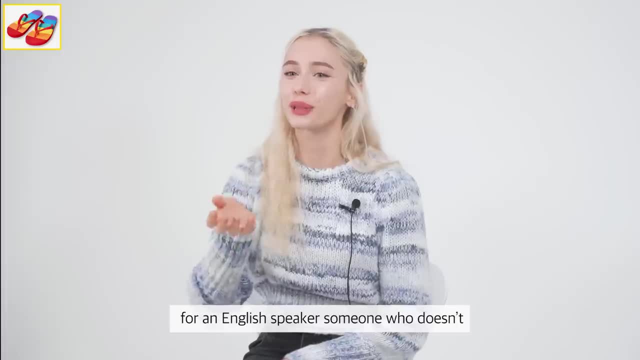 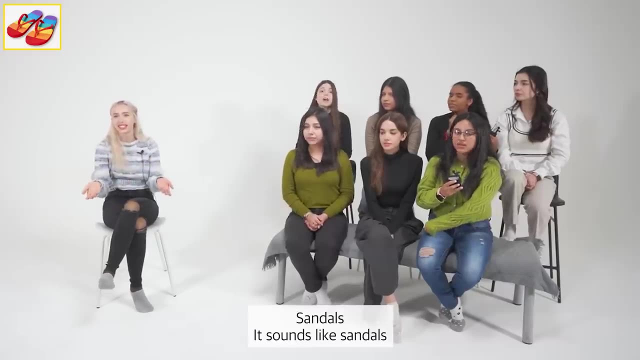 Yeah, that's true, The power of the chancla. For an English speaker, someone who doesn't study Spanish, They would recognize sandalita- sandalias, I think, Because it sounds like sandals And actually we also have sandalias in Spain, But it's more for those cute open shoes for summer. 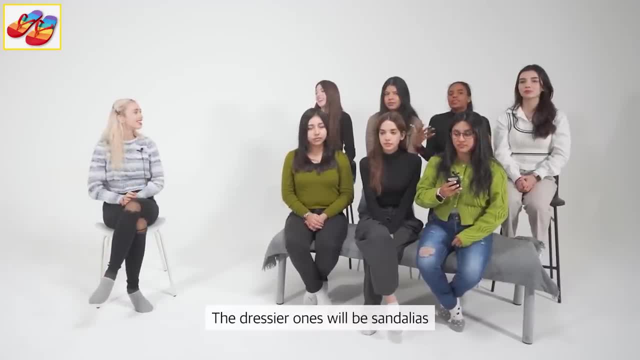 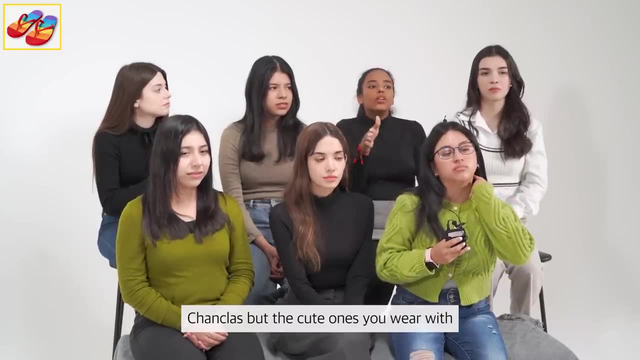 Yeah, the nice ones, The rubber ones, would be sandalia And the one that, like you know, like Havaianas, Yeah, yeah, yeah, Like the plastic one, like Havaianas, Those are chanclas, But like the cute ones you wear with dresses and stuff are sandalias. 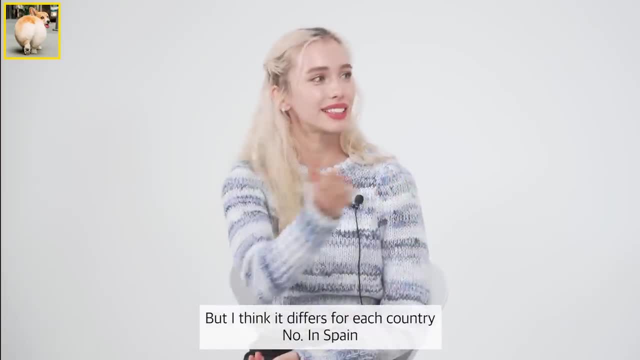 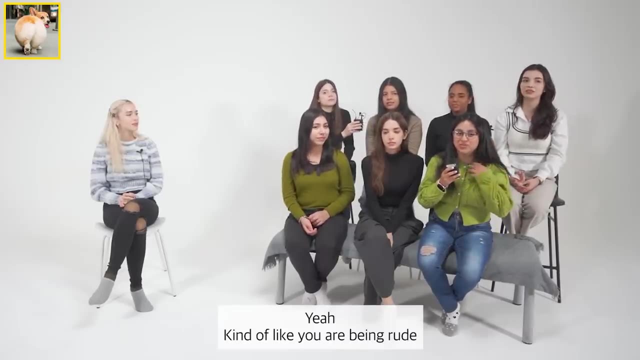 So in English we would just say butt, But I think it differs for each one. No, in Spain Culo, But for us, like culo is such a strong word. Yeah, Kind of like you're being rude. Yeah, it has that feeling. It's more like for, like, reggaeton songs. 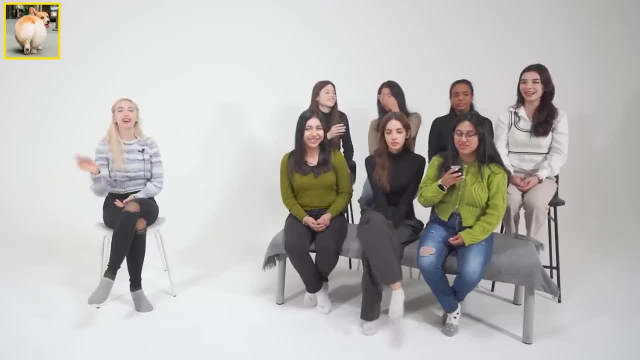 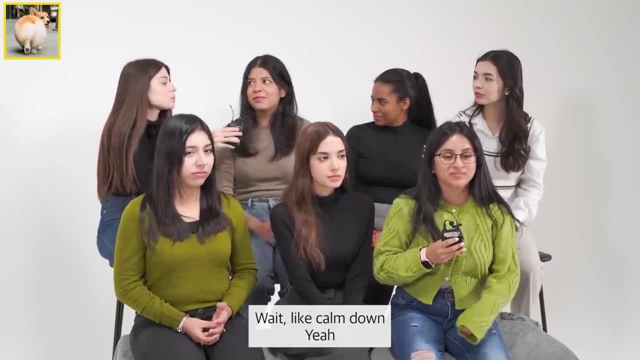 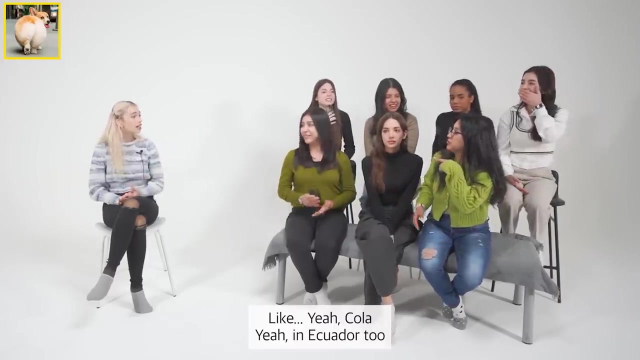 Yeah, In Mexico, I don't know, we have many words. We have like trasero, Yeah, but I think culo is like wait, like calm down. Yeah, In Colombia we say cola, Cola, Like cola, You're better too. Cola actually means tail. 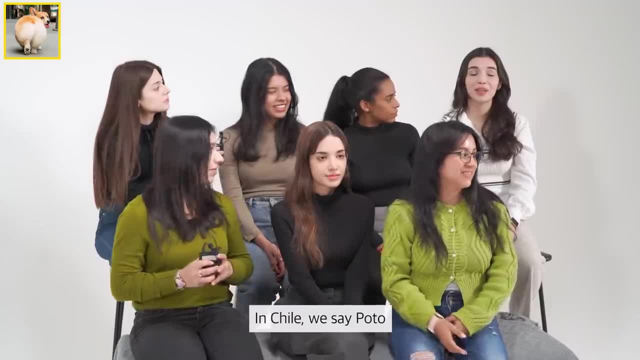 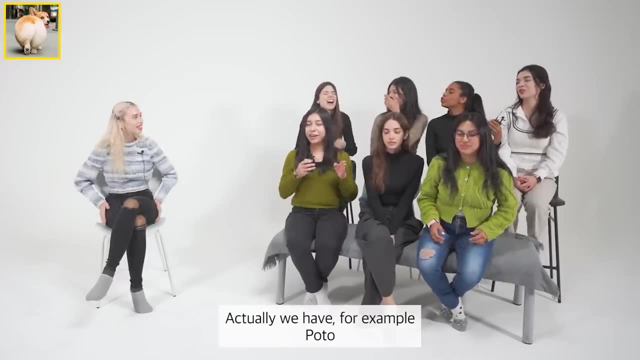 For real. So it's like: Yeah, Ah, okay. In Chile we say poto Poto, Yeah, yeah. In Peru we say poto too, Like bata Poto. Actually we have Pot Pot for example. Oh, poto Poto, yeah. 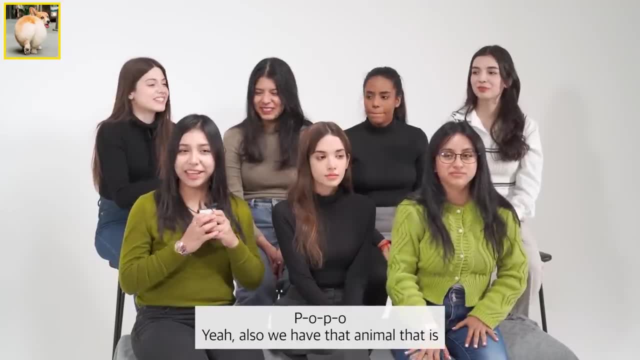 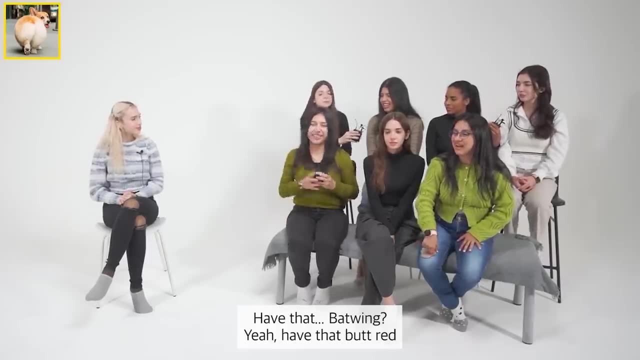 P-O-T-O, P-O-T-O, Yeah. Also, we have an animal that is mono poto rojo. Because, Is that true? Yeah, Yeah, If you want to say it like, like, strongly, You can say culo or las nalgas, Like Nalgas. 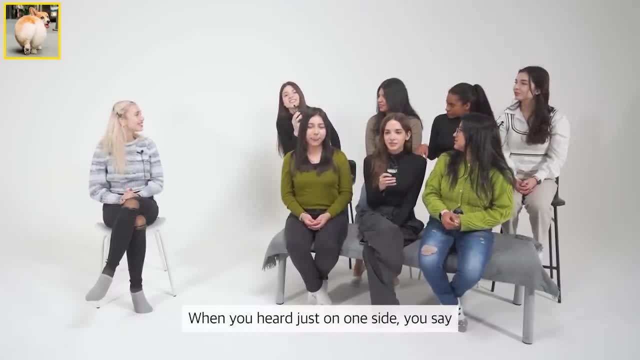 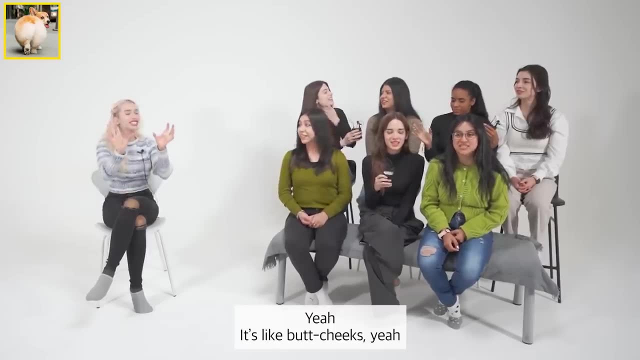 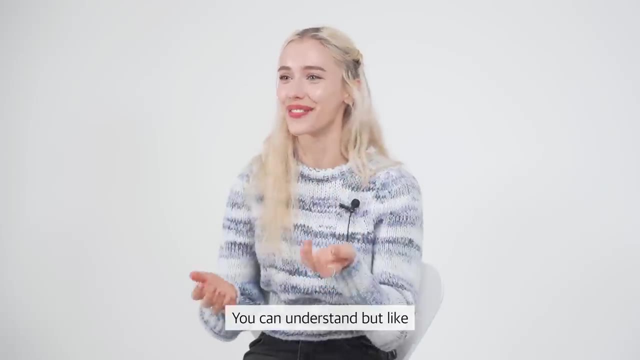 Nalgas. Yeah, when it hurts just on one side, You say la nalga izquierda With nalga is cheeks. Yeah, Yeah, Yeah, Oh. this is really fun. It's so it's funny to watch them like all laugh at each other Because, like you can understand, 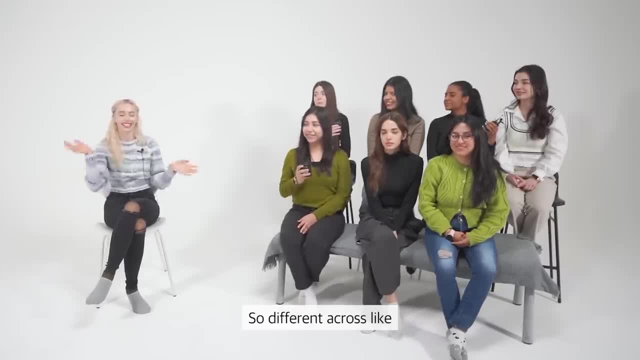 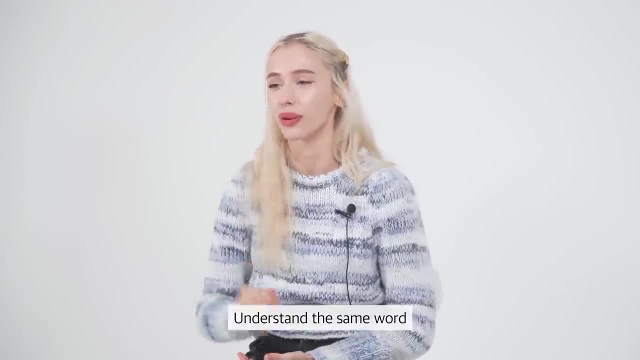 But like the meanings, like we've explained, are so different Across like across the world and in different countries and stuff. So it's really fun. It's really interesting for me Because now I know a bunch of different ways to understand the same word. Actually, I feel a little bit out of place.